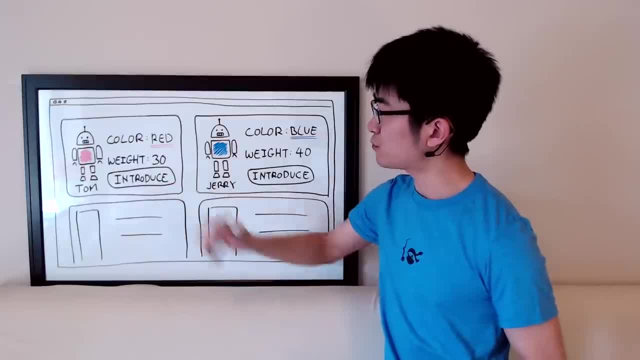 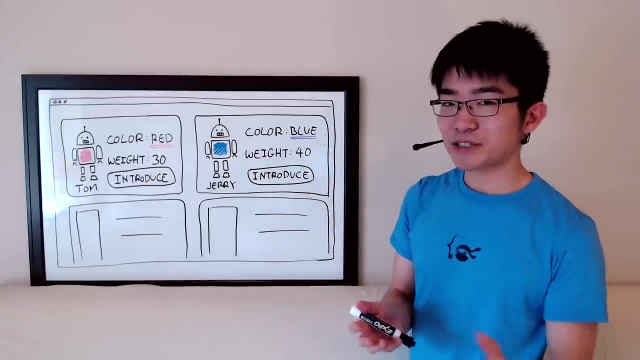 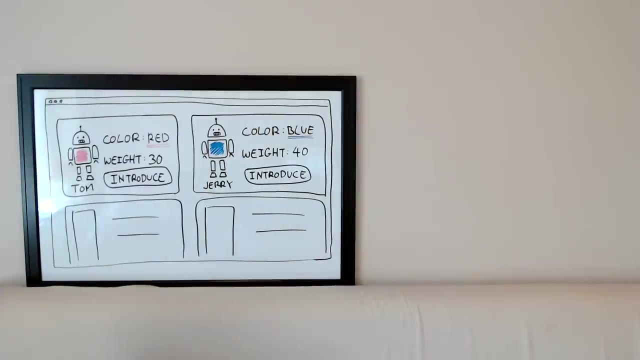 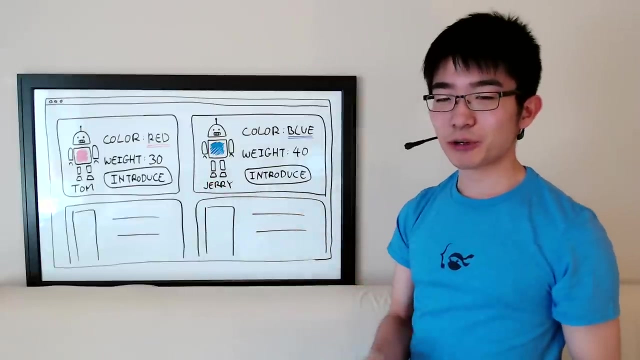 so they are a little different. So when this button comes up, it's like the same thing. You know, when you click this button, introduce Tom will say my name is Tom and Jerry will say my name is Jerry. And that's all you have for now, And it's pretty basic, but that's all you want at the beginning when you create this website. Now, to create a system like this, you basically need a way to represent these different entities or these different robots in whatever programming language you're using, whether it's Python, Java or JavaScript, And that's where the 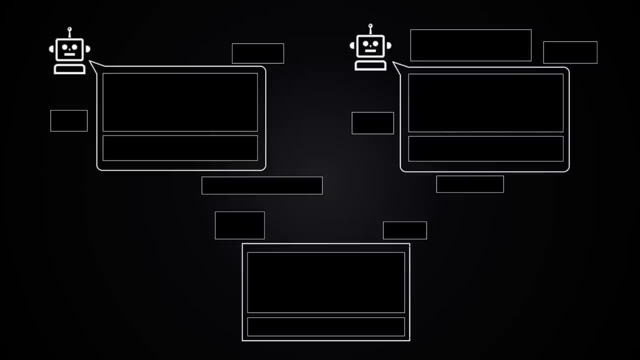 classes and objects. come in now to represent each of these robots tom and jerry that we saw earlier. in whatever programming language you're using, you need to store two sets of information. the first set of information that you need to store is the properties that each robot has, so, for example, the 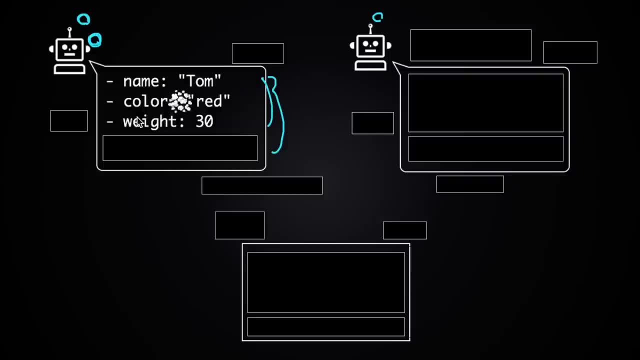 first robot we saw had these properties. its name was tom, the color was red and the weight was 30 pounds. and the second set of information you'll need to store for each of these robots is the set of functionalities it has. as we saw earlier, it had only a single functionality in. 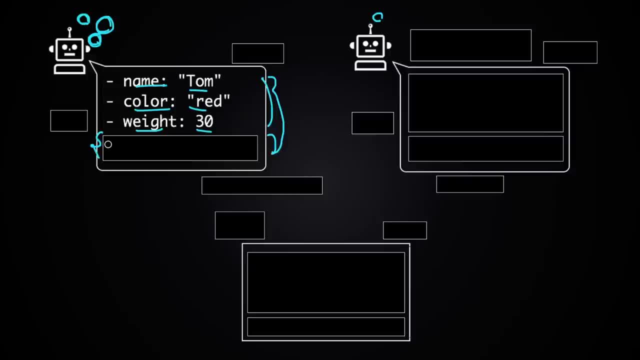 this particular case and that was to introduce itself and that might be represented as a function in whatever programming language you're using, and let's just call it introduce self here for now. at this point you might say, is there any convenient way to organize these properties and functions together? 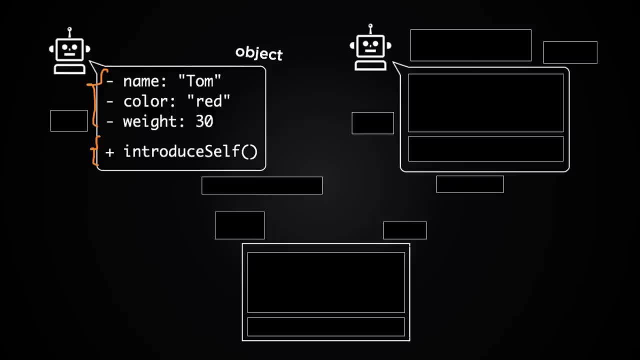 there is and that's called an object. an object is basically a collection of properties which can be expressed as variables and some functions, and with that collection of information an object can represent something, whatever that thing is. so in this particular case, this particular object is representing this particular robot tom. but you can make an object so that it represents a particular 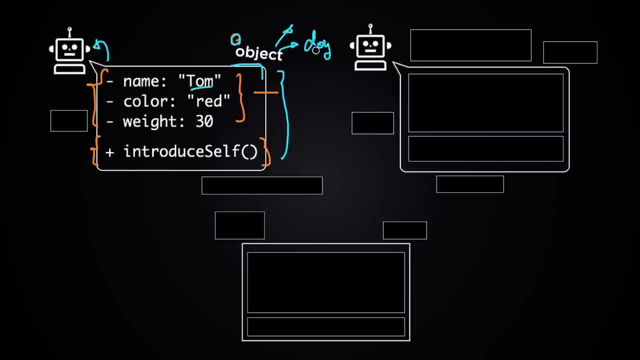 person or a particular dog or anything else for that matter. if you decide to represent a particular person with an object- let's say lady gaga, just as an example- you might have a different set of variables and a different set of functions to represent that person. so, for example, you might 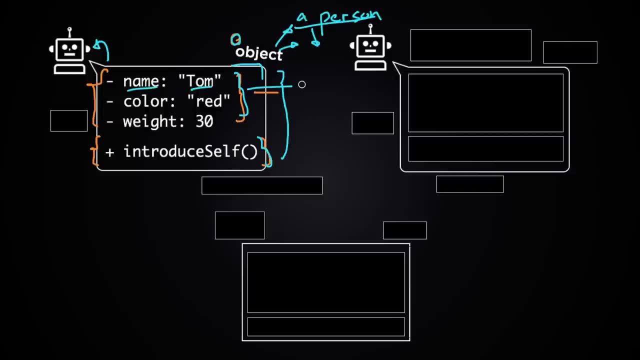 still have name, but you might also have height and weight, eye color and ethnicity and so on, and your object will probably have a different set of functions too. let's now go back to the final part, to look at shooting this robot. and now let's go back to right display, and every time you have an object, resourcelet's a variety of. 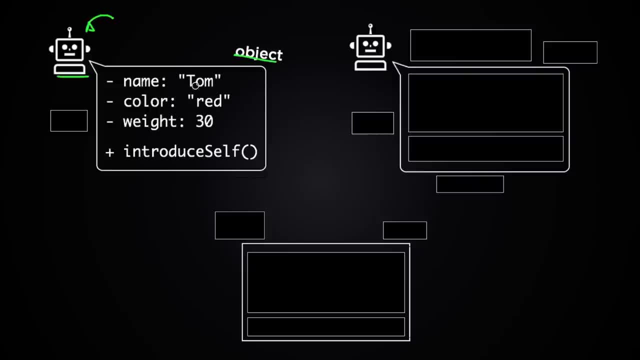 variables. you can set up everything individually. you're going to have a whole database of a variety of different things, and actually one of them is the things that are necessary for each of the variables. but here you've got a list of all of the elements and traffic that you want to run, and also. 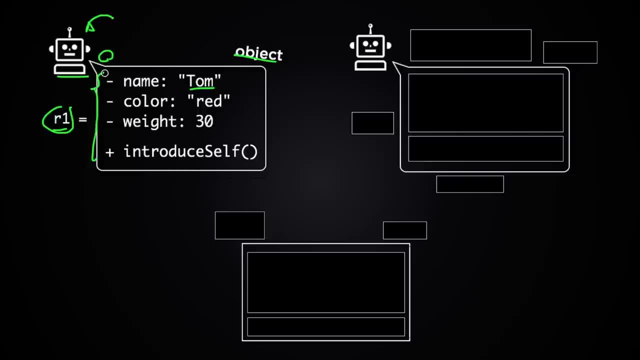 that contains this whole set of information. you know the properties or the variables and the functions just like any other variables, for example, to pass it into a function as one of the arguments. okay, let's now take a look at how the second robot we saw, jerry, can be represented. 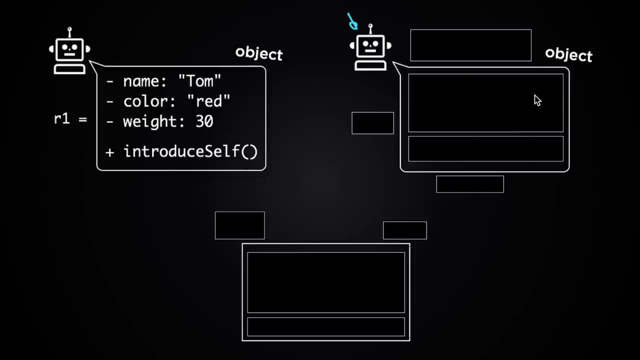 with an object, it's going to look pretty similar to the first one. it's going to have the same set of properties, but different values- this time jerry, blue and 40- and the same function as well. introduce self. and, of course, once you create this object, you'll be able to put it in a variable as. 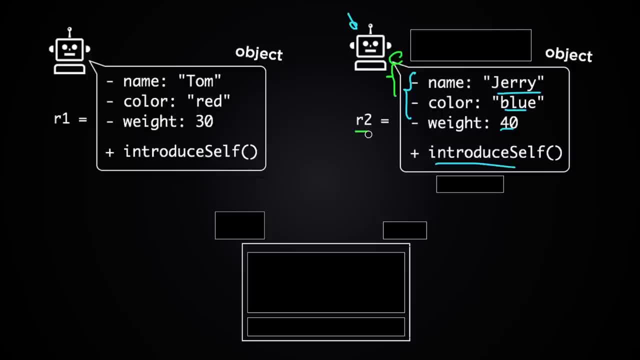 well, let's call that one r2. and because you have two distinct variables containing two different objects, you'll be able to distinguish them very easily in your code. and just quickly about terminology: these variables within an object are called either instance variables or attributes, and these functions within an object are called 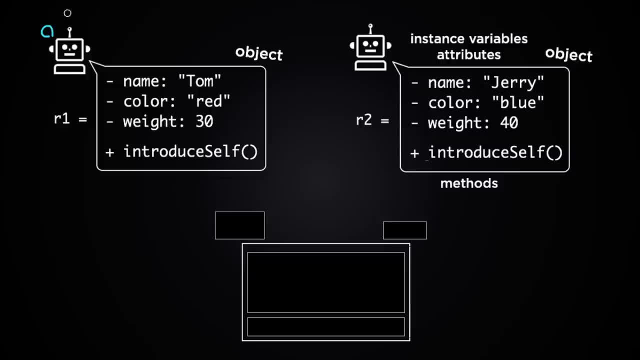 methods. okay. so when you see these two objects you might say, well, they're pretty similar. they have the exact same set of variables or attributes and they have the exact same set of functions- only one function in this case. so you might say, is there any convenient way to organize that somehow there? 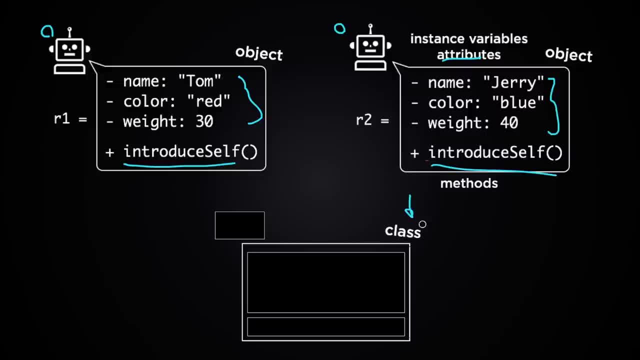 is, and that's why we're going to call it a set of variables and we're going to call it a set of class variables. okay, so if we have the set of ones, it's going to be the first of those and look like, and what kind of properties should it have and what kind of functionalities should it? 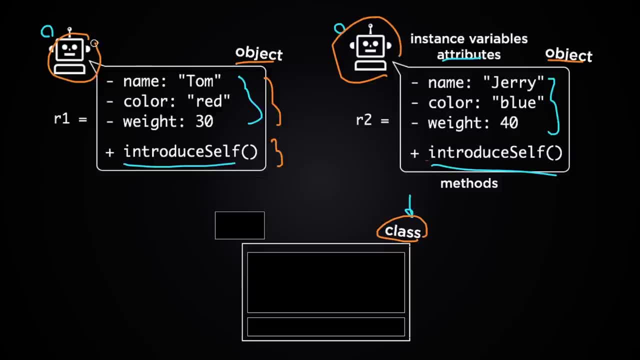 have. So basically, if you want to make a robot in sort of the real world, you'd need a blueprint to make the from, to know what the robot should look like. And that's sort of how it works with programming, with objects and classes too. So when you make an object you'll want to know what kind 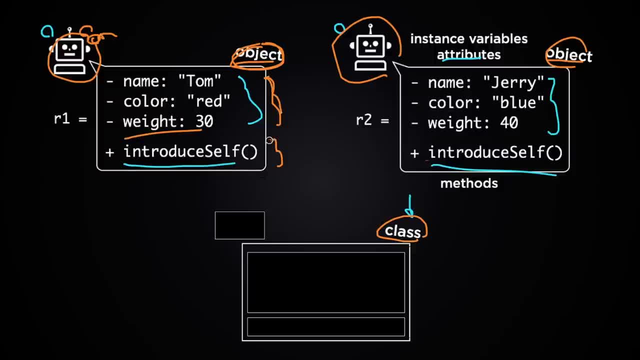 of properties, what kind of attributes it'll have and what kind of functions it'll have, And you can use a class to specify exactly that. Okay, let's now see what this particular class might look like for these two objects, these two robots. It'll probably look like this: As you can see, it has. 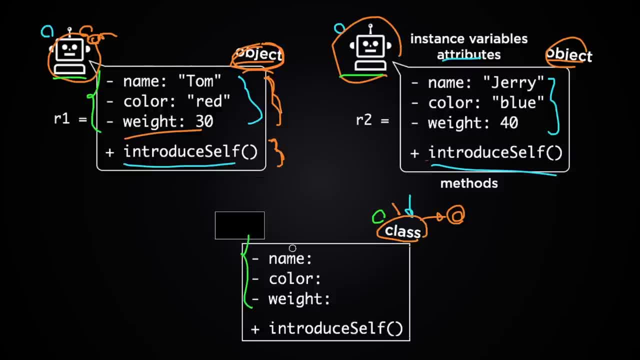 the same set of properties as the objects themselves: name, color and weight. But the values for these three properties are not defined yet, And that's because a class doesn't refer to any particular object. It doesn't refer to this robot or this. 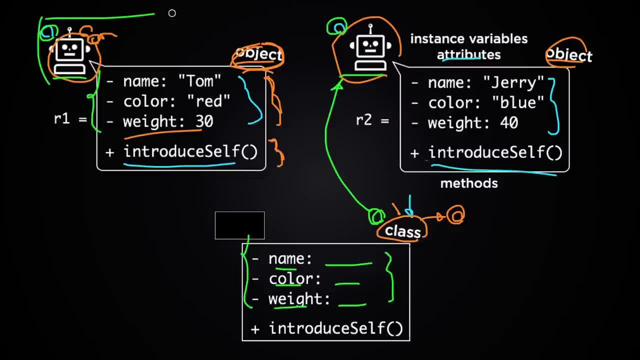 robot in particular. it just refers to this category of robots or this type of robot in general, and then when you create a specific object using this class, then you can specify what the name should be, what the color should be and what the weights should be, and also notice. 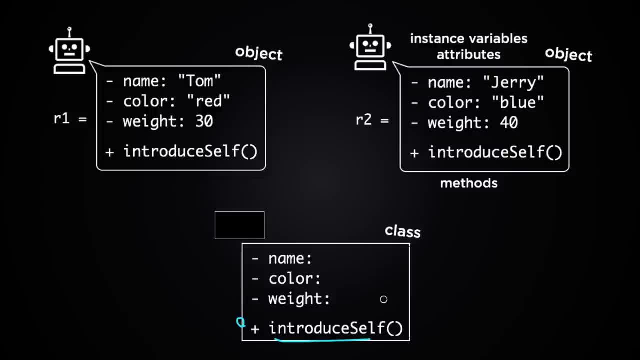 here that we already have the introduce cell function in this class and you can actually implement it already when you define this class by writing something like this. so this is just an example from java. in java, for printing something on your computer, we have systemoutprintln. it's similar to the print function or the printf function in other languages, and then inside the 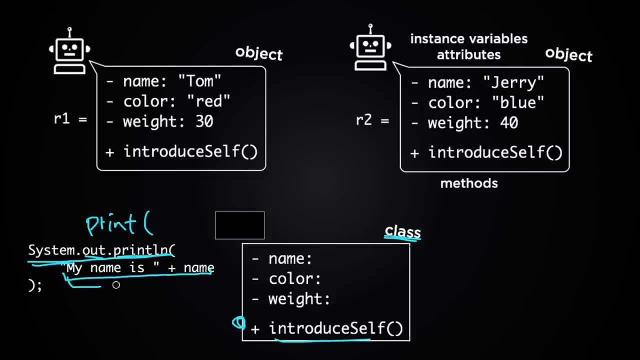 input of this function. we have my name is as a string plus name and this name will refer to whatever the value of the name is for that particular object. so, for example, if you run this function in this object, it's going to print out: my name is tom, because that's the name. 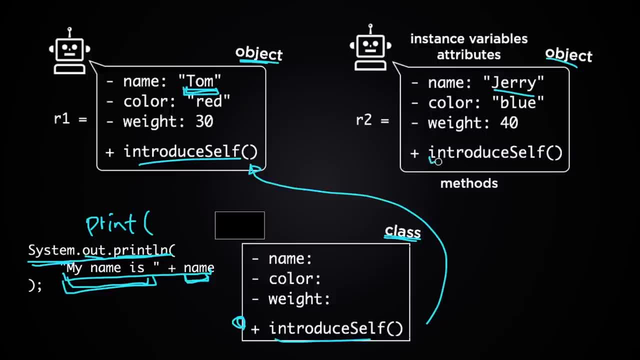 of this particular object and then if you run this function here in this object, instead, it's going to print out: my name is jerry instead. and one more thing to note here is that when you define a class like this one, you need to give it a name. it could be anything, but let's call it robot here. and, as you can see, 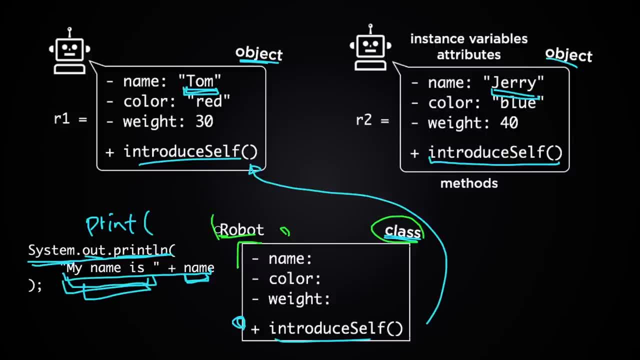 the first letter, r, is capitalized, and that's a pretty common convention when you name a class. okay, let's now take a look at how this whole thing might look like in code. we're going to take a look at some code in java here, but other languages are typically pretty similar, and let's 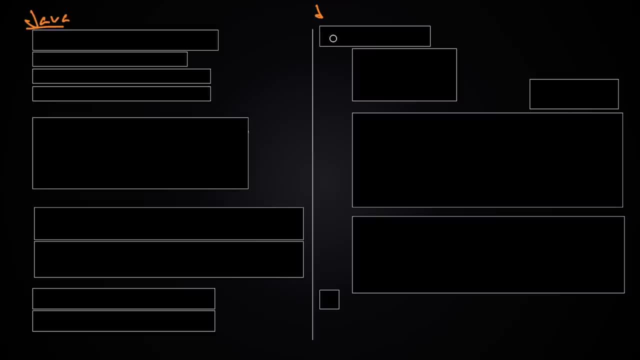 first assume that we already have our class defined. like we said, it's going to be called robot, but we're going to take a look at what's going to go inside later- and once you define this class robot, you'll be able to use this class, of course, to create an object out of it, and you can do that. like this, we have robot. 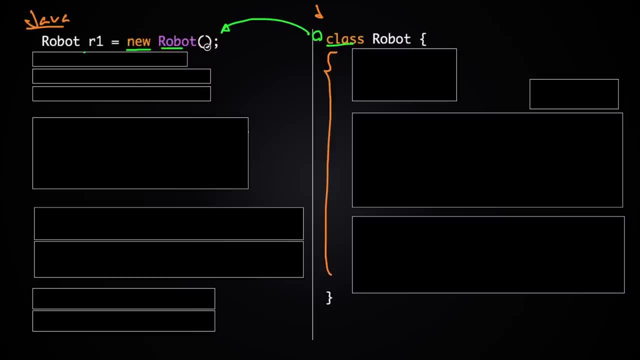 r1 equals new robot, and this new robot- parenthesis- says: create a new object with this class robot, and then we're assigning that object to r1, and then we have the word robot again, because a class is used not just to create an object but also as a type two. You know just. 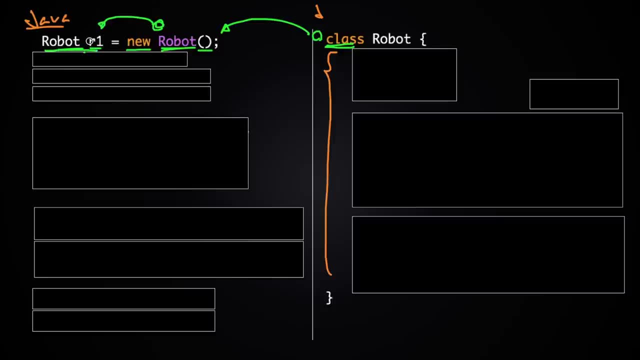 like we say string R1, if we want to create a string, we can say robot R1 to create a reference to a robot object. Okay, let's move on. When you create a new object this way, this new object doesn't have the properties, doesn't have its instance variables set yet, So you need to set. 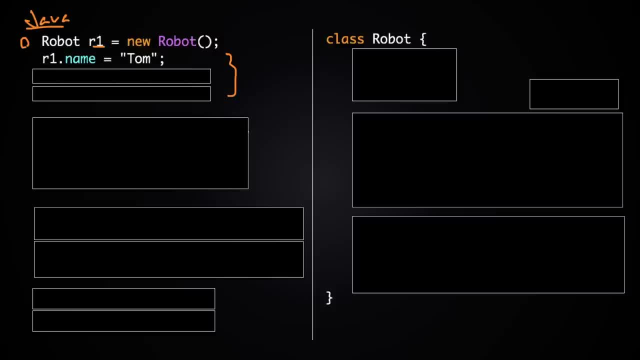 them after that, just like that, Here we have R1 dot- name equals Tom, And that sets the name attribute of this object or the name instance variable of this object to Tom. And then you need to do the same thing for the other two instance variables, by saying R1 dot- color equals. 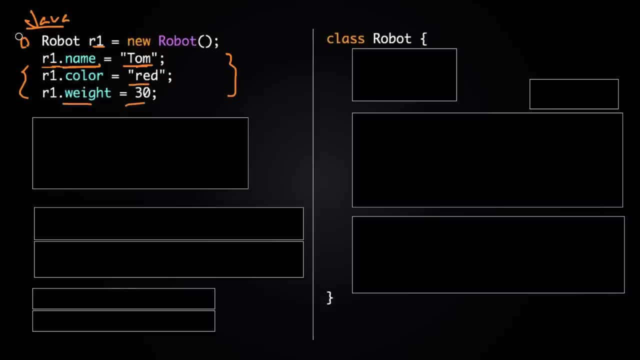 red and R1 dot weight equals 30.. So that's the first object, R1.. Let's see how we can create a second object here. As you can see, the second block of code here is the first object, R1. And here is pretty similar to the first block. we have robot R2 equals new robot. to create a new. 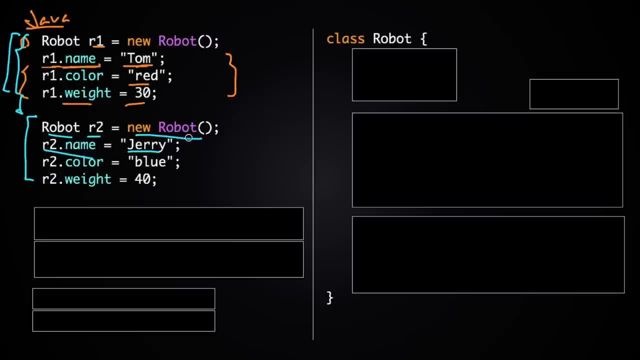 object And then we have R2 dot name equals Jerry and so on to set the instance variables of that object. So that's how you can create two objects of the robot class here. But what about the functionality we saw earlier introduce self to run the function for each of these objects? 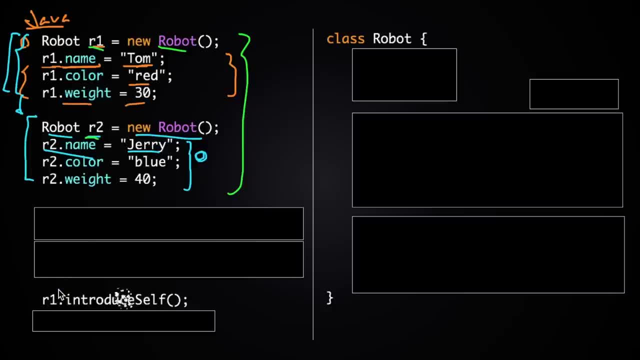 the syntax for that is actually pretty simple. It's going to look like this: R1 dot- introduce self. This just says: run this function, introduce self on this object R1.. So when you run this line, it's going to print out: my name is Tom, because this robot's name is Tom. 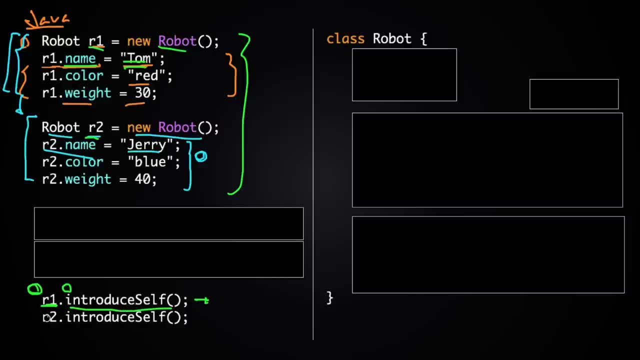 And then you can do the same thing for R2 by writing R2 dot- introduce self. And that's going to run this function: introduce self for R2.. And then it's going to print out: my name is Jerry. Okay, let's now see how you can create a second object: R1 dot- introduce self. So let's go ahead. 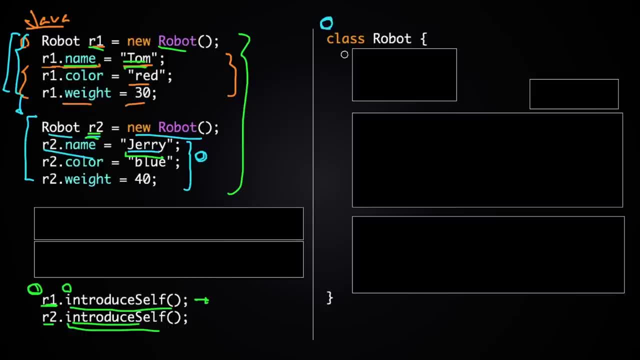 and run this function, introduce self And then you can actually define this class. First of all, to define what instance variables this class will have, you can just write these. This, of course, says the instance variables that this class will have: our name, which is going to be a string color. 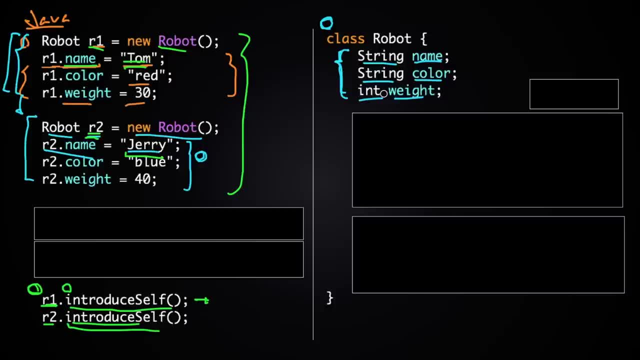 which is a string as well, And weight, which is an integer. And when you see other sample code in Java, you might see words like public, private or something else before each of these attributes. But just to keep this simple, I'm not going to talk about what they are in this particular tutorial And when you run this code, 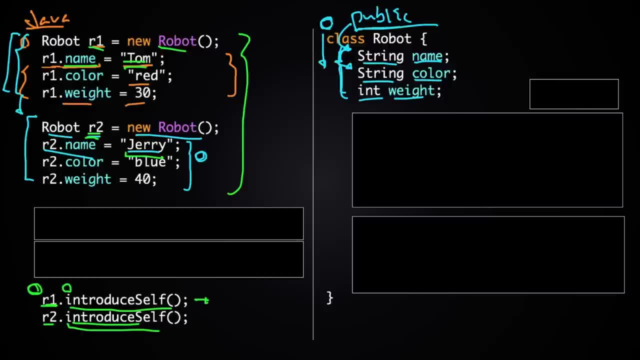 it will just work just fine without adding these words too. Okay, the next thing you need to define and implement is this function, introduce self, And for that you can write this Here: we are defining a function called introduce self, And we have the void prefix here to show that this. 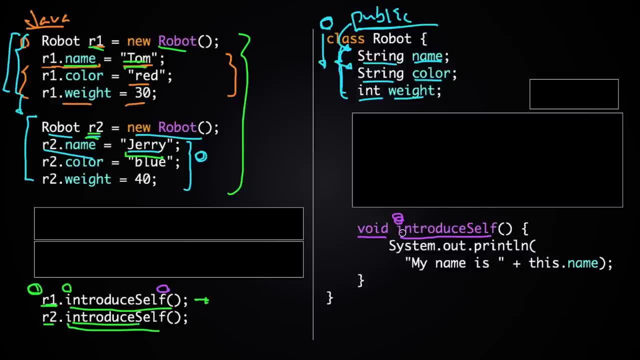 function is not going to return anything And notice that this function definition is still inside this class, And then the implementation is, as we saw earlier, systemoutprintln. my name is thisname. Actually, we could just have name here, But I wrote thisname instead, just for emphasis. So what's this? 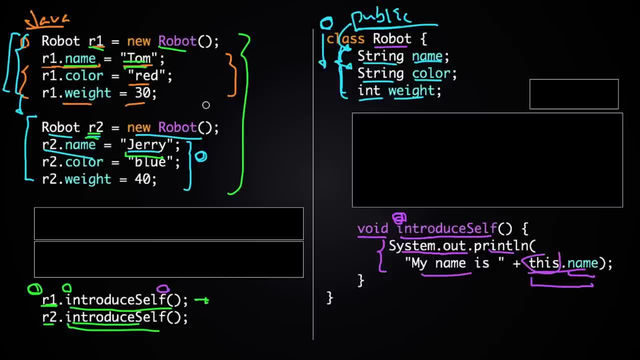 here. this refers to whatever object, whatever particular object that you're running this function on. So if you write r1.introduce self, you're running this function on r1. So this will be equivalent to r1. So it's going to be sort of like saying systemoutprintln. my name is r1.name, which is going to be. 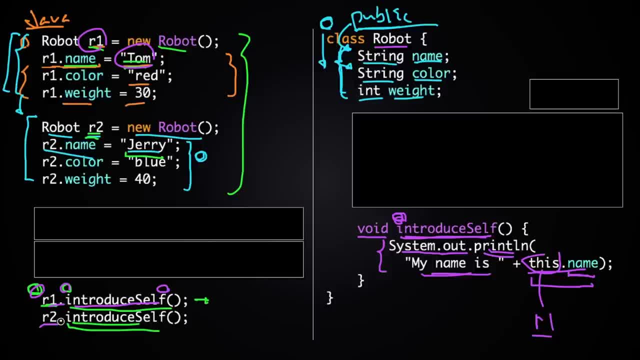 Tom, of course. And then when you run r2.introduce self, this will refer to this keyword, will refer to r2 instead. So when you run r2.introduce self, it's going to print out my name is r2.name. 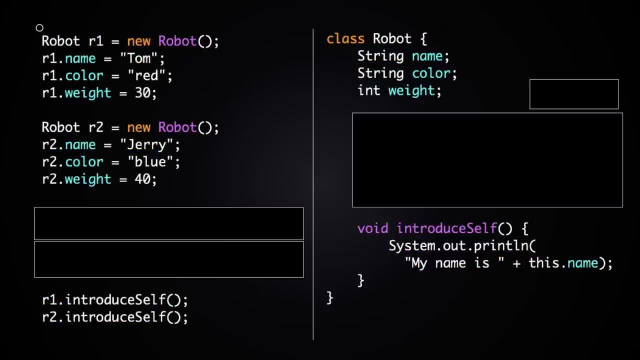 which is Jerry. Okay, so that's the basics of classes and objects in Java. But when you look at these two blocks of code you might say, Well, they're pretty repetitive. you know you need to repeat the same things over and over again And then it's pretty cumbersome to remember to set. 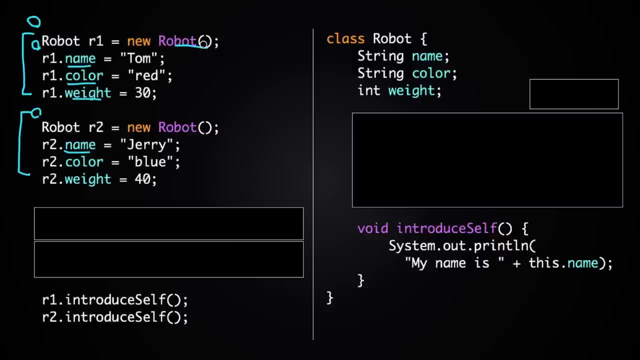 these attributes every time to every time you create an object. So you might say, Is there any way to simplify that? there is, and it's called a constructor. a constructor is basically a function that allows you to create an object from a class, And then you'll be able to use the constructor to 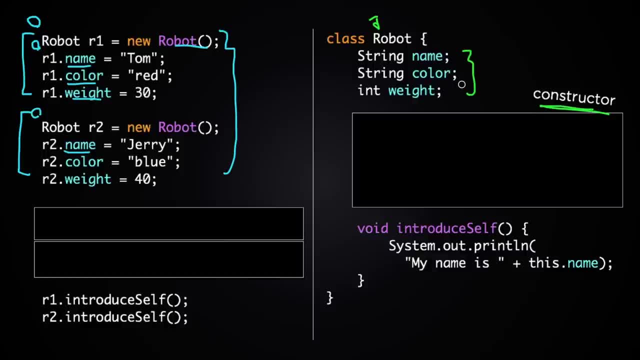 you know, do things like set the attributes for yourself and actually you already used a constructor. you know this line right here: new robot, that's a constructor, but that's a default constructor that java defines for you, and this constructor doesn't set any of the attributes. so let's see how we can create our own constructor that does set the attributes for you, so that 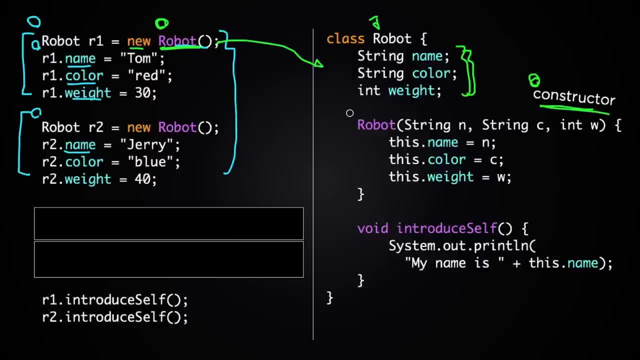 constructor might look like this. so if you see this function, you notice that you know it looks like a regular function, except for that we don't have any prefix here, like void or string for the return value. instead, this function, this constructor, is just called robot. notice that that name is. 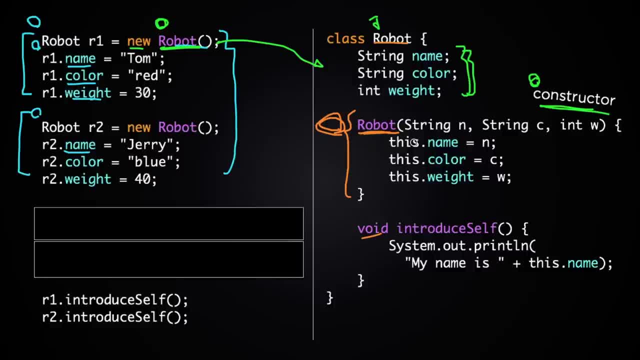 exactly the same as the class name, and then it has three arguments: string n, string c and int w. and then inside this function we're setting this, not name to n, this the colored c, this that way to w, as we saw earlier. this we've added a function here which refers to the particular object that we are talking about here. 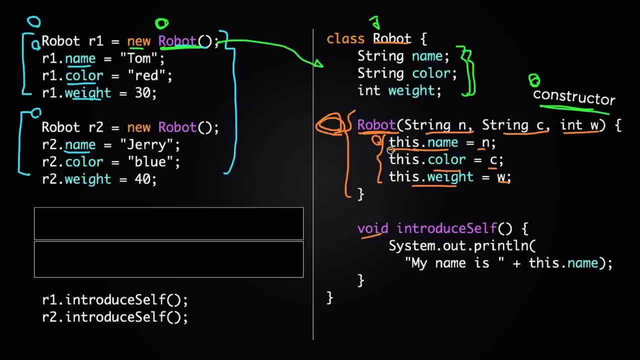 in this case the particular object that has just been created. and then we're saying that object's name should be n, which is the given argument, and then that object's color should be c, which is the given argument, and so on, and then here the common practice here is to name these arguments exactly. 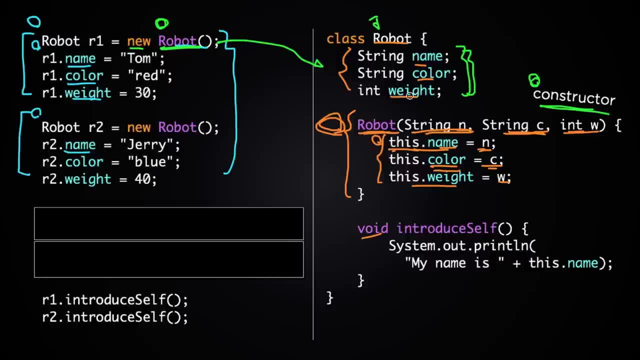 the same as these attributes- name, color and weight- and with that this part is going to look like this: dot name equals name. that color equals color. this that weight equals weight. but with that naming this function, this constructor is doing exactly the same thing as this one, so that's really just a style issue. 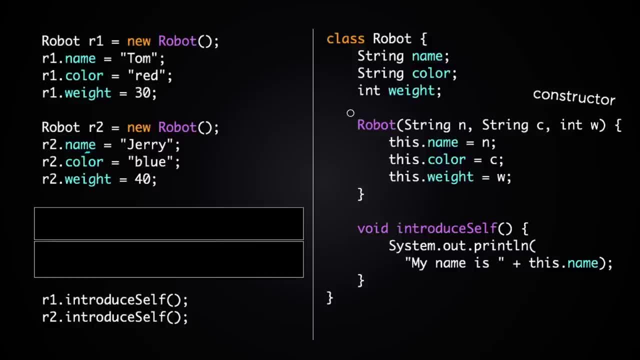 okay, moving on, we're almost done here. let's see how we can actually use this constructor. and actually, when you define your own constructor, your own custom constructor, the default constructor stops working. so these two blocks of code no longer works, and then you can use this new constructor to create new objects, just like this. this one says robot r1 equals new. 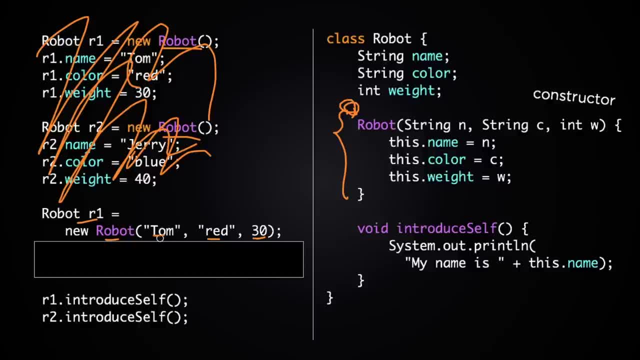 robot, tom, red and 30. so these three arguments- tom, red and 30- will be passed on to this constructor, and then this block of code is going to be run, and so r1's name is going to the given n, which is tom, and then the color will be red and then weight will be 30. 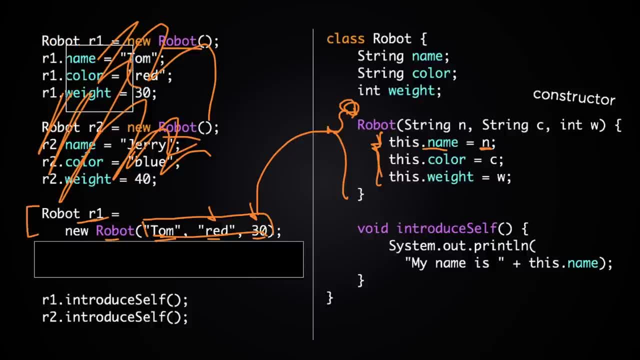 so this piece of code will actually be equivalent to the whole block of code we had earlier right here: basically create a new object and then set the attributes to the given arguments, and then we can do the same thing for r2 as well by writing robot. r2 equals new robot, jerry, blue and 40. this 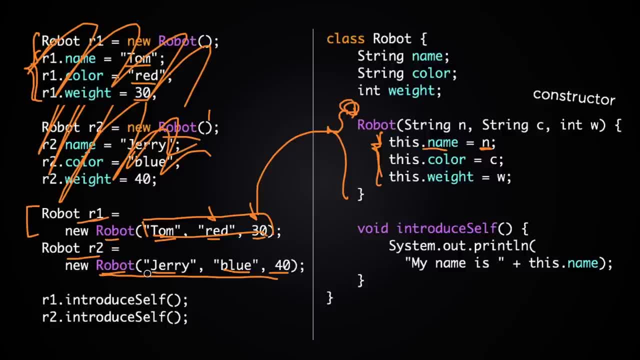 creates a new robot object with the name jerry, color blue and weight 40.. and after creating these two objects, you'll be able to use r1 and r2 just like before, by writing r1.introduce self and r2.introduce self. okay, again, this was just sample code in java. 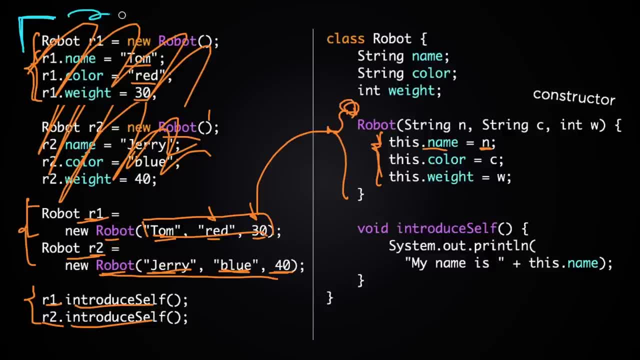 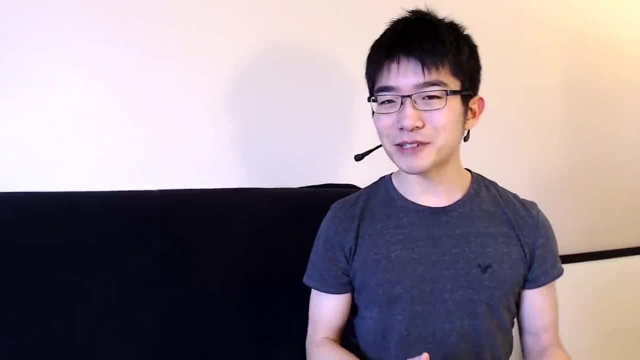 but it's pretty similar to other languages too, and you'll be able to find links to sample code in both java and python in the description below. all right, if anything was unclear in this video, please let me know in a comment below, so maybe i can talk about it in the next video. 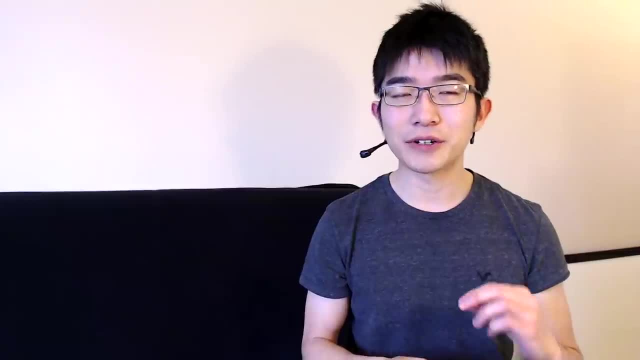 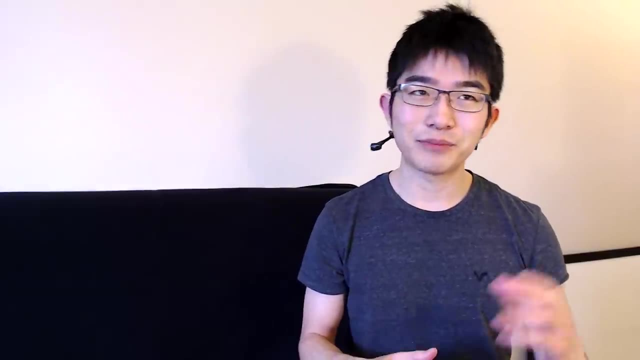 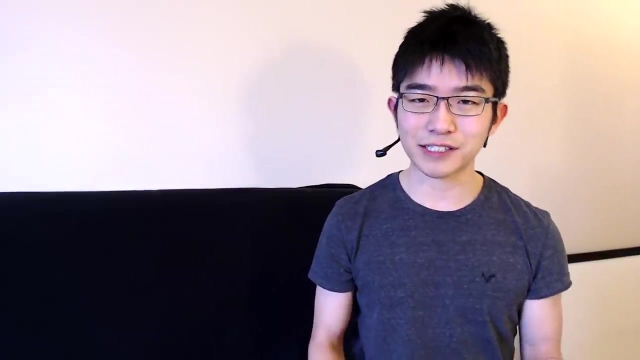 in the next video i'm also going to talk about how you know multiple classes and objects can interact with each other, and with that knowledge you'll be able to finally start building some data structures like linked lists. i'm also planning to create a new python tutorial video on classes. 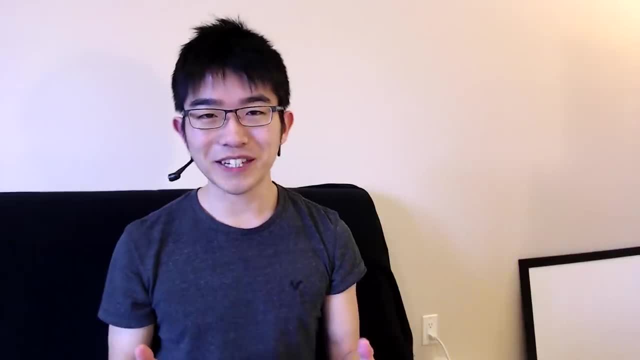 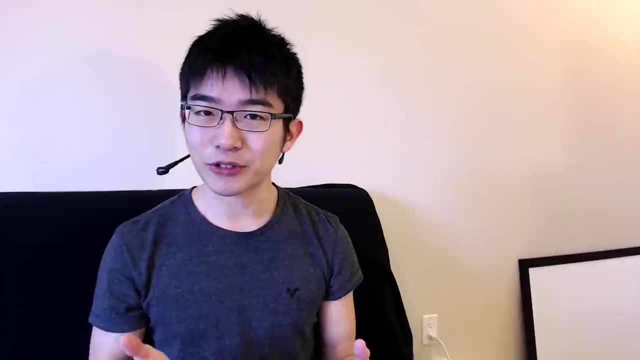 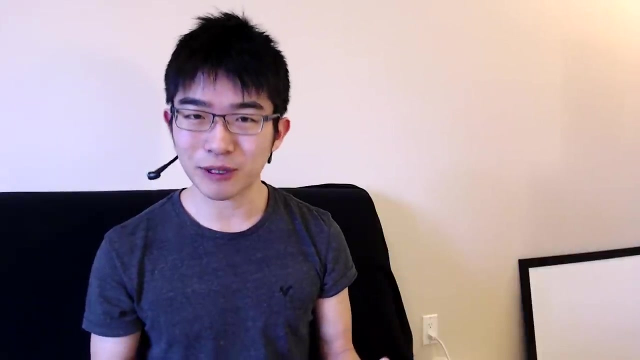 and objects, so look out for that as well. and special thanks to brilliant Mediator for sponsoring this video. you know some of you may already be familiar with data structures and algorithms and, as sort of a refresher, If that's the case, brilliantorg might just be the right website for you to learn more. 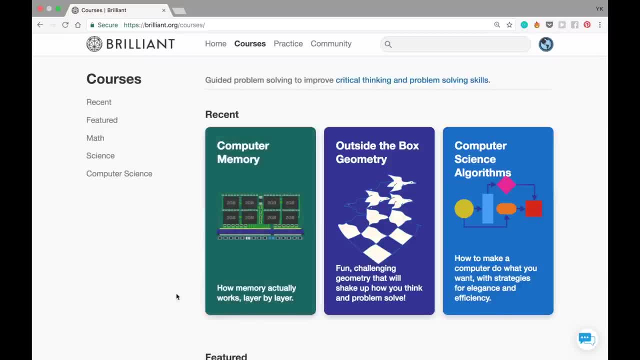 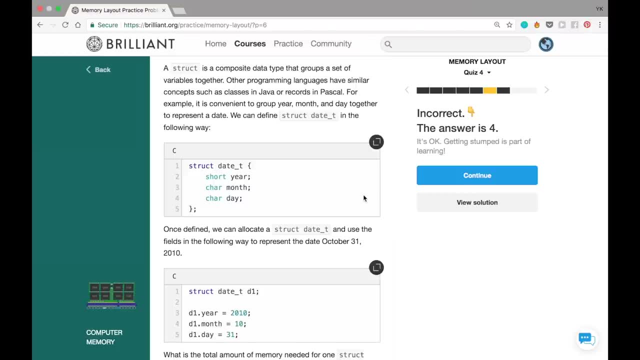 advanced concepts in computer science. So personally I use this computer memory course to get a better understanding of how memory works in a computer. For example, previously I didn't really know how structs in C are stored on memory. I mean, I had a vague idea but I didn't really know. 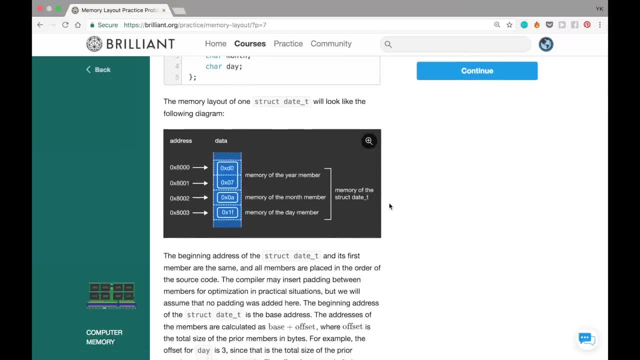 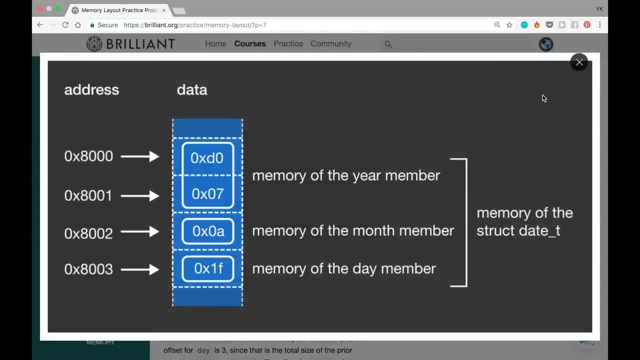 And I found this course was really helpful for understanding that. Personally, what I like about Brilliant is, first of all, the fact that they have really nice visuals, like this one- you know, much nicer than mine, I would say- And they're helpful for understanding different concepts visually. 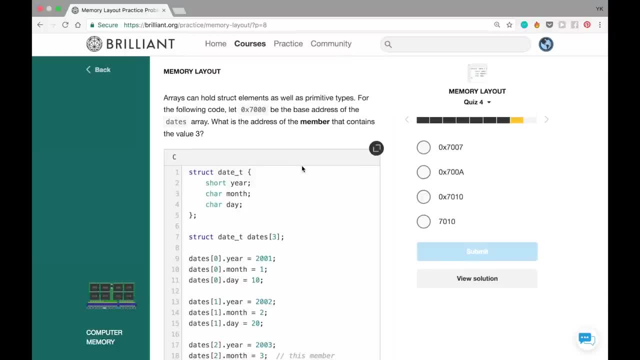 And another thing I like is the fact that they sometimes combine multiple concepts in a single problem. What I mean by that is, for example, for this particular problem, you need to understand different things like binary expressions and how structs in C are stored on a computer. 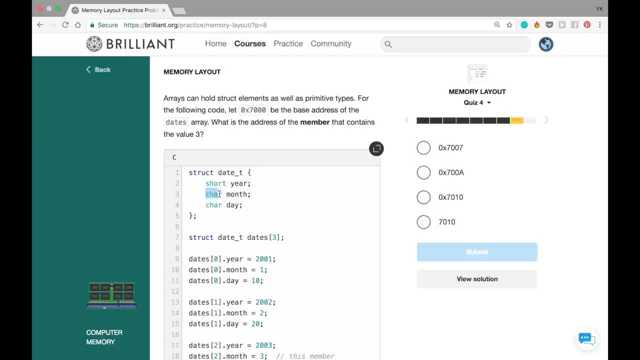 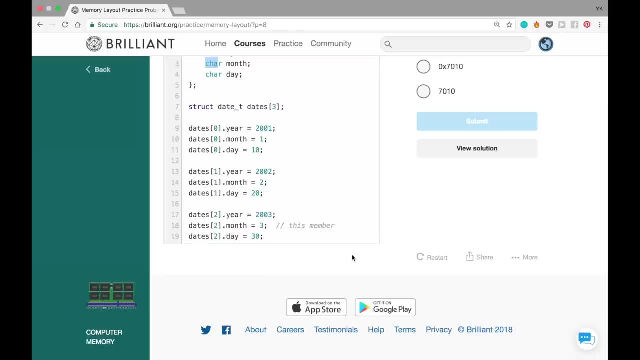 and how short and char And different types of data are stored on memory too, And in my experience in general, I have found that, you know, solving problems is a really good way to review different concepts at the same time and also learn new concepts. 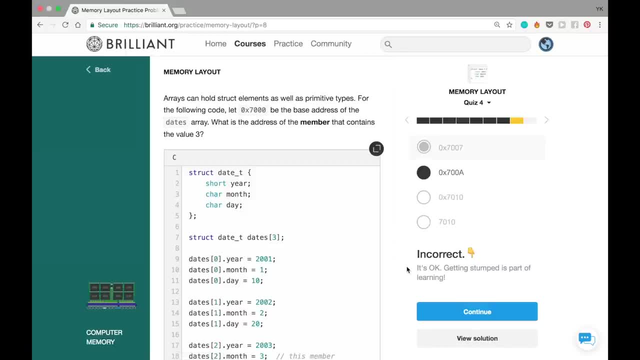 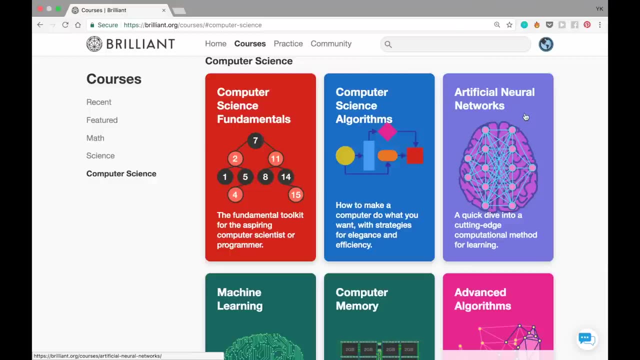 And brilliantorg definitely does a good job of coming up with good problems to solve And they even have pretty advanced courses, like this artificial neural networks course, on top of their standard computer science fundamentals and algorithms courses. You can just go to brilliantorg. 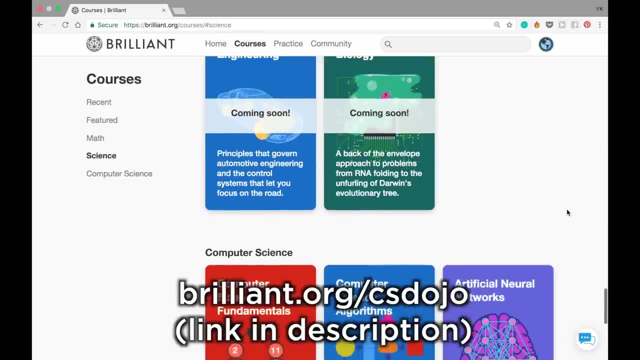 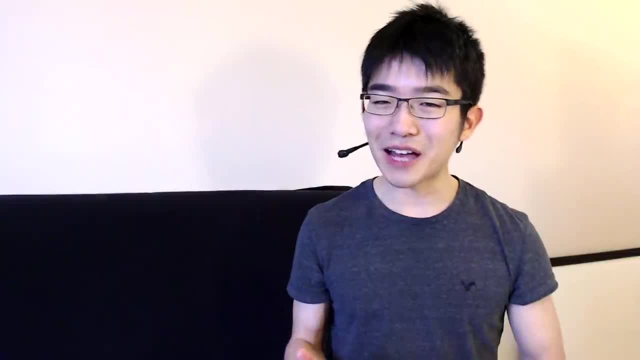 Slash CS Dojo to start checking out these courses yourself, And you can get a 20% off their annual subscription through that link as well. Alright, as always. I'm YK from CS Dojo and you know I'm working really hard here.